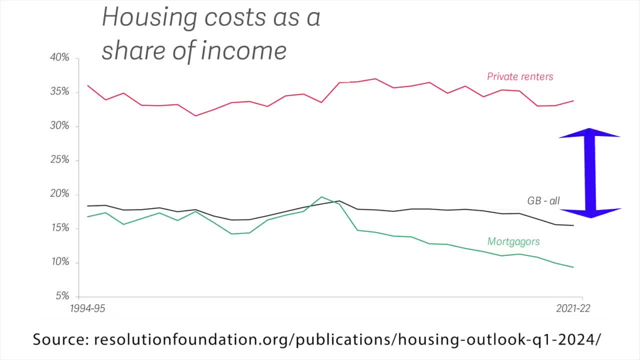 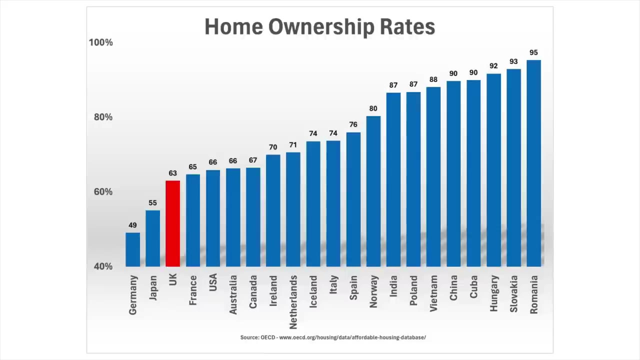 cost between private renting and owning with a mortgage. there's a big difference between the two models. This is why people strive and strain to take out a mortgage. but if we look at international comparisons, the UK home ownership rates are actually quite low. Home ownership rates peaked. 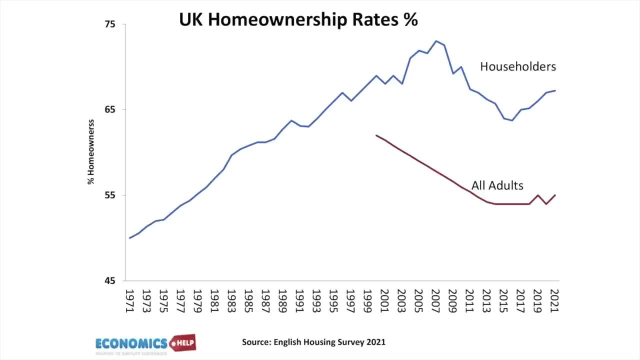 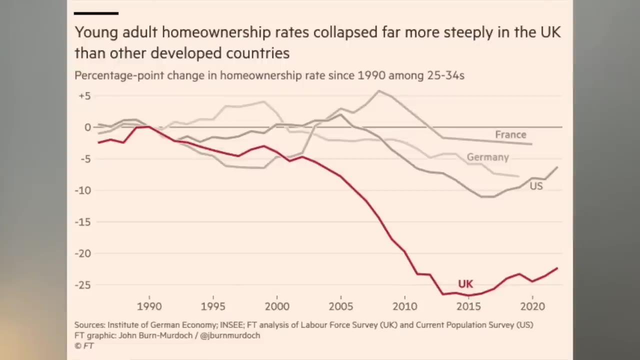 around 2007 and have been in decline ever since. And if we measure home ownership rates by the percentage of adults rather than households, the rate is even lower because many young people have been forced to live with their parents or in bigger shared housing, And the UK has seen the 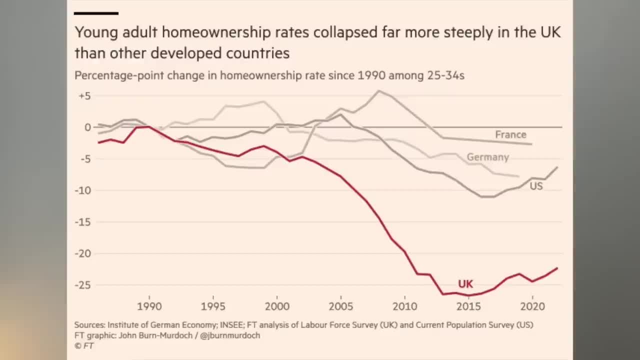 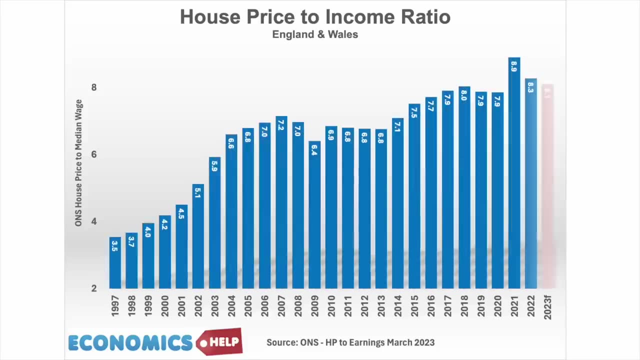 biggest slump in home ownership rates amongst the young, compared to many other countries. The simple problem is that housing as a share of income has increased dramatically since the mid 1990s. It's currently running at a ratio of eight times income and in many major cities such as. 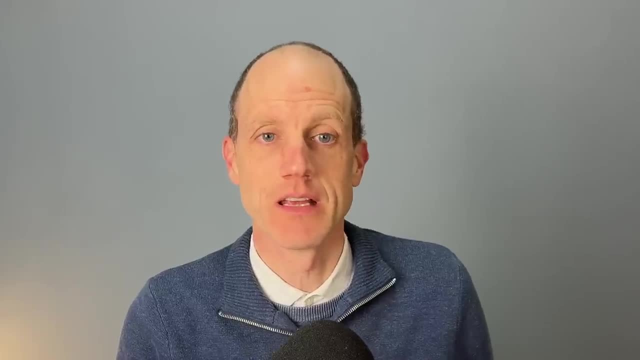 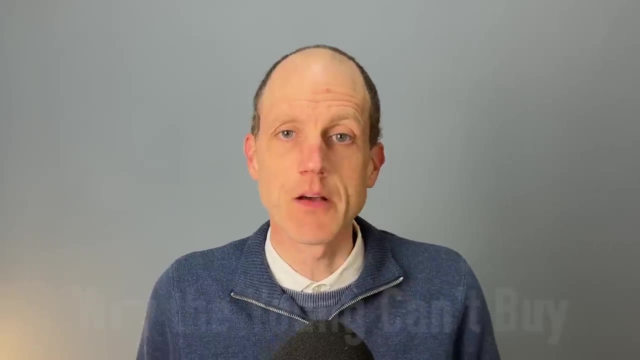 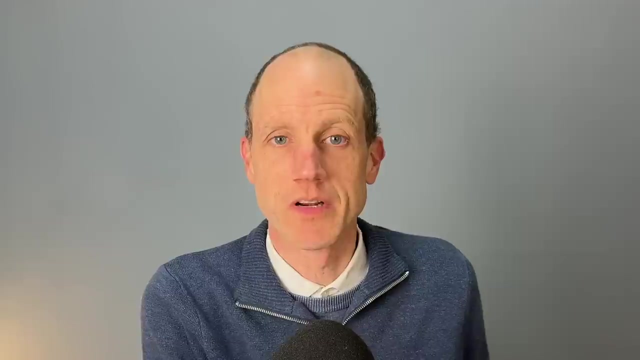 London and Oxford and Cambridge. it's over 10 times income And there's been only a very modest improvement in affordability since the 2022 peak. Now, since the credit crunch of 2008, there has been new mortgage regulation to try to prevent the abuse of high mortgage multiples and there's 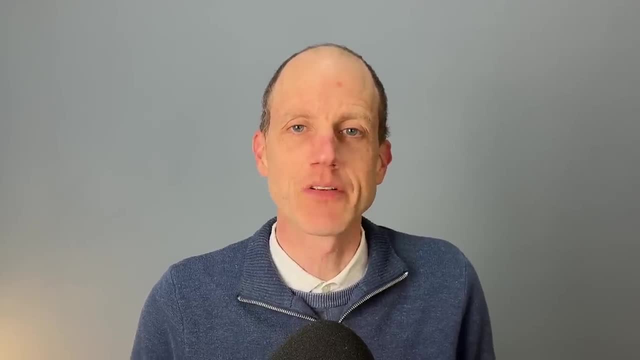 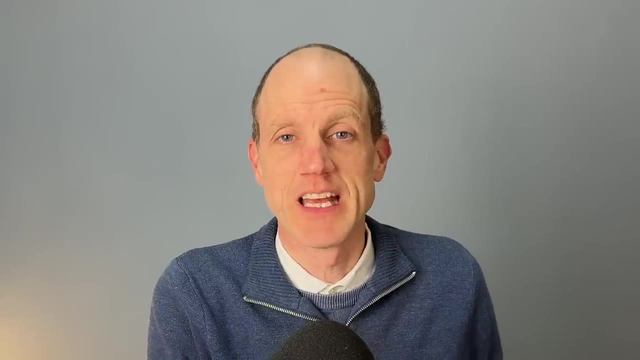 better stress testing. What this means is the housing market is now in a position where it's more likely to be able to afford more. It's somewhat more resilient to higher interest rates, but also that young people find it much more difficult to buy, even if they would like to get away from a private rented sector. With median 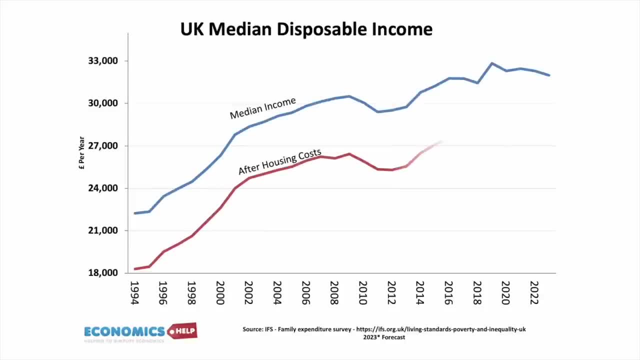 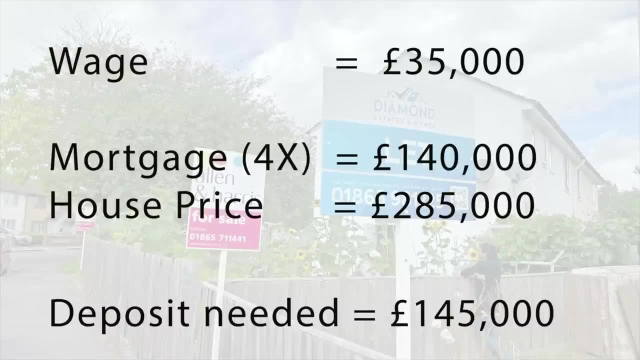 salaries running at only £35,000 and barely increasing in the past decade. a standard mortgage multiple of four times income leaves a young worker struggling to get anywhere near current average house prices. It's not just about housing costs, but in recent years we've seen a squeeze on 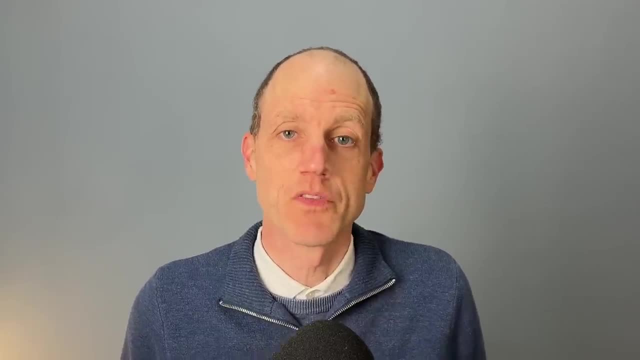 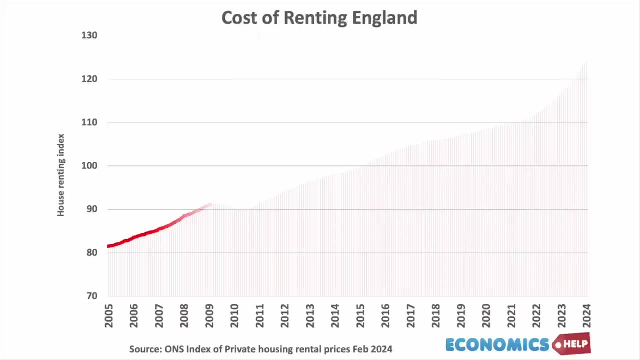 dispensaries. We've seen an increase in the cost of housing for young people. We've seen an increase in the cost of housing for young people. We've seen taxes rise as a share of GDP, plus the burden of student loans for young graduates, And then, on top of that, we've had a record rent increases And the rise in rent. 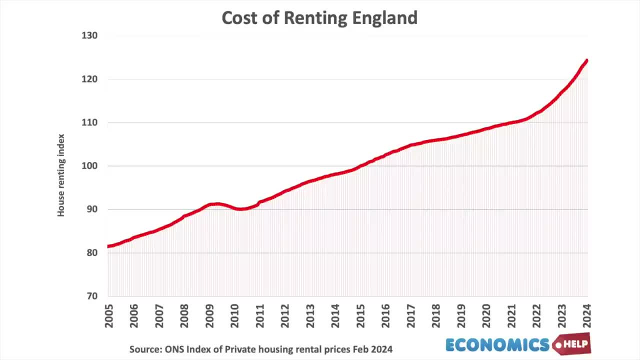 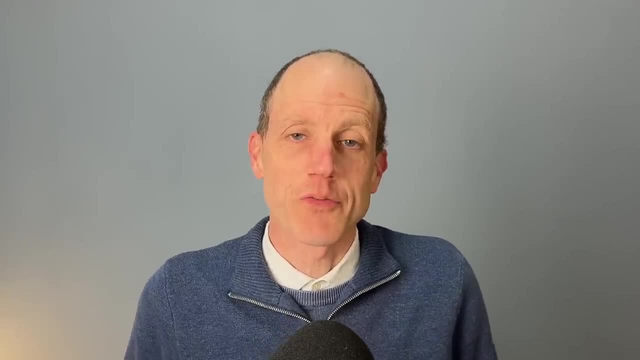 is not always fully captured by CPI because they use an imputed value. But the main problem the UK has is we've had very low growth in real wages, whilst house prices and rents continue to rise. The result is that unless you have a very high income, you're not going to be able to afford. 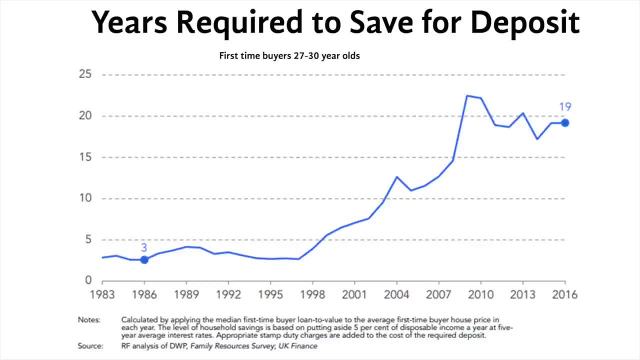 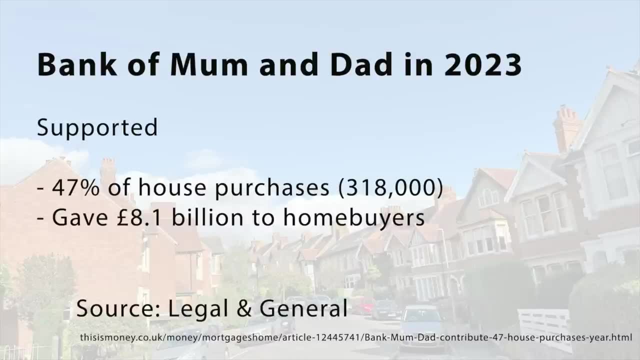 to pay rents And if you have a very high income, parental wealth to help with deposit has become almost a key requirement for getting on the property ladder. The UK has become more unequal, with a bank of mum and dad supporting 47% of home purchases in 2023. 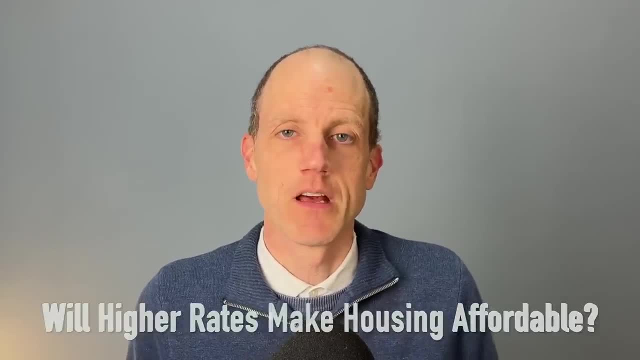 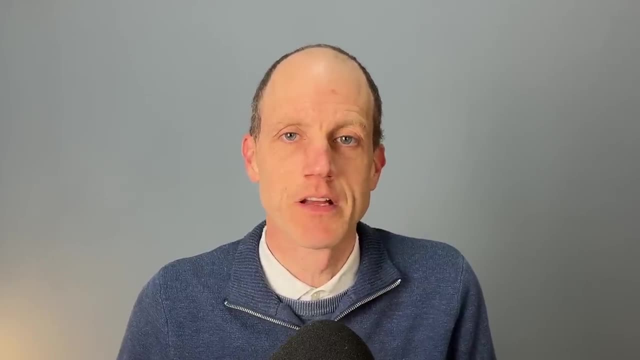 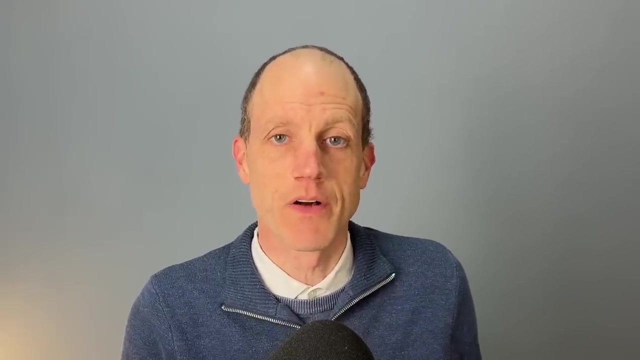 Now for those who did manage to buy, especially recently. the recent rise in interest rates have caused a shock, with mortgage payments rising as a share of income to high levels. In sectors like buy to rent, we've seen arrears rise 50% as many struggle with a higher mortgage. 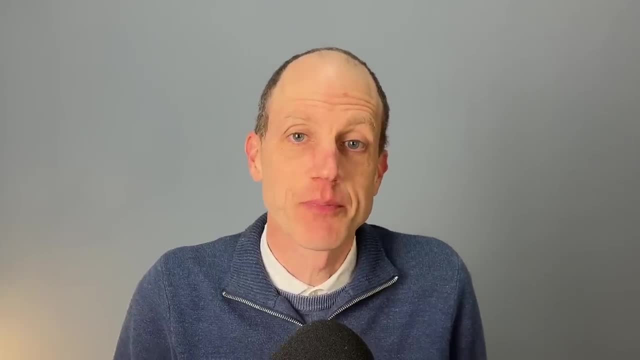 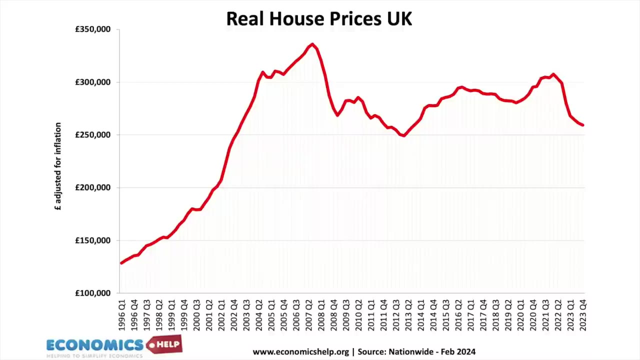 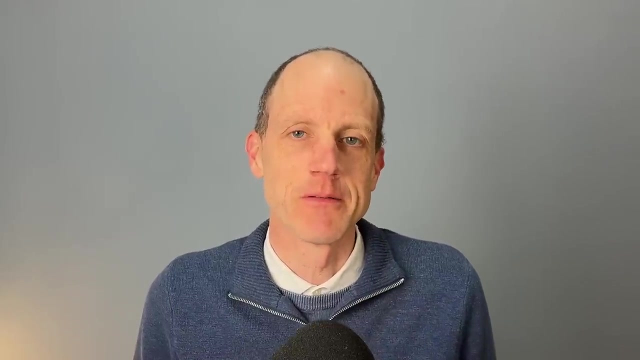 payment. Now, the effect of high interest rates has been to slightly improve mortgage affordability, with a 14% fall in real prices since 2022. But the average buyer is yet to notice any real sense that buying a house is affordable like it was in the most of the post-war period. 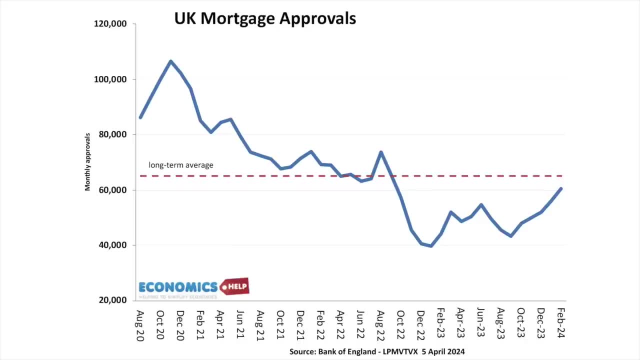 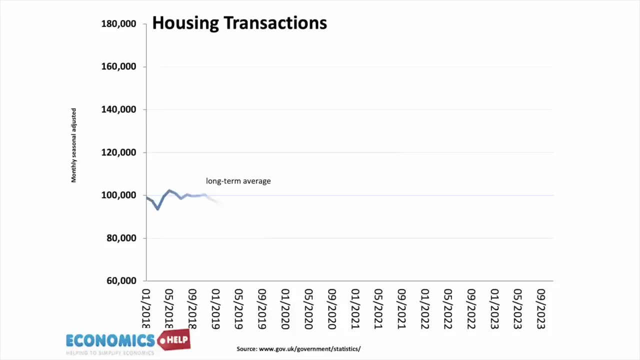 Now, last month mortgage approvals did rise, admittedly from low levels, but it is a sign that activity is returning to the housing market after a period of very low property transactions. Now there's also been an increase in homes for sale and this perhaps explains the to some unexpected fall in prices. 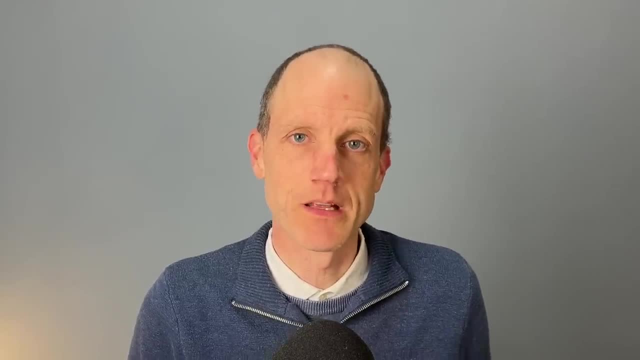 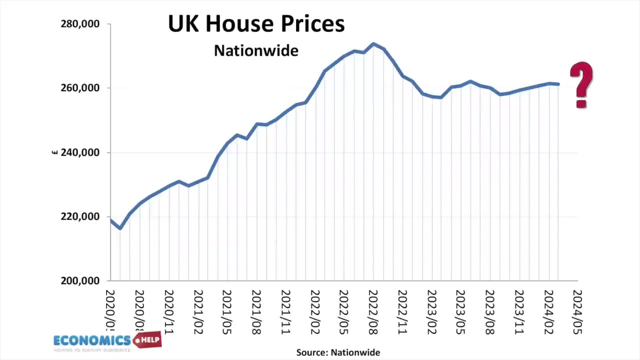 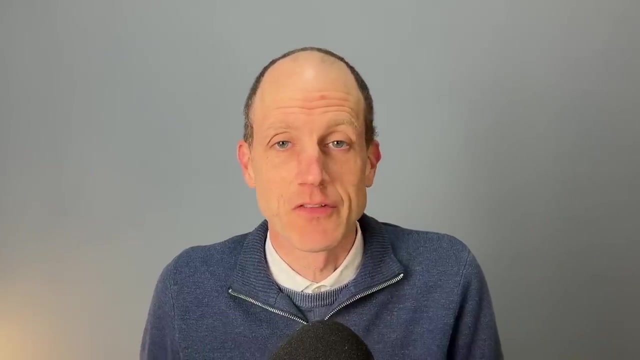 last month, reported by Halifax and Nationwide. But this all raises the question of whether the past six months is just a temporary bounce in prices or a sign that a much needed correction is probably as much as you can expect and there's no prospect of further falls. Because if demand can be increasing in this climate of high interest rates, recession and low income growth, there's really no hope that UK housing will ever become affordable. However, before we herald a new chapter of house price growth, it is worth bearing in mind there is good and empirical evidence that house prices historically react to higher interest rates with a time lag. 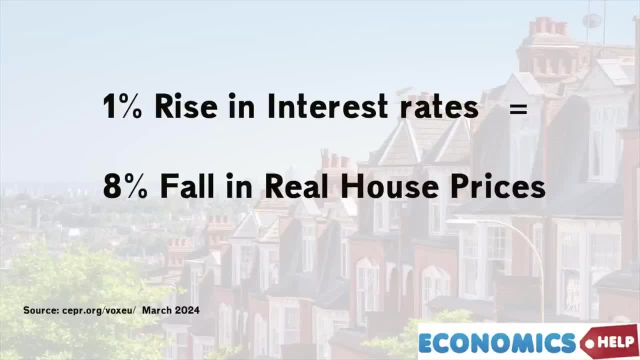 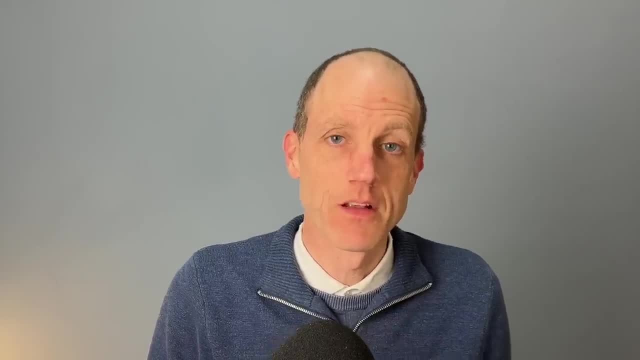 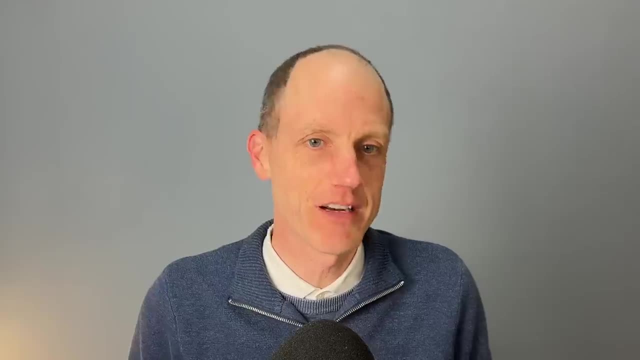 Now one OECD study found that a 1% rise in interest rates causes an 8% fall in real- that's inflation- adjusted house prices. So with the UK having nearly 5% rise in interest rates, that's in theory a 40% fall in real prices. And even if interest rates were to be cut back to 4%, which is likely by the end of the year. that would be an 8% fall in real prices. It would still indicate that some house price falls are to come. Now for those who are sceptical about the prospect of any further house price falls, 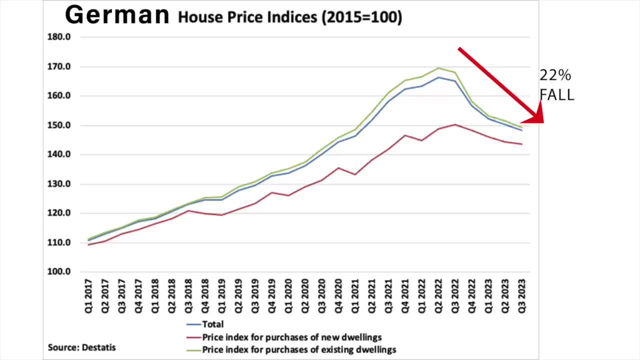 don't forget this study was based on real life examples. For example, in Germany, house prices have fallen 20% since their 2022 peak. That's around 35% fall in real terms. Now is the UK housing market so different that it is impossible to predict what will happen in the future. 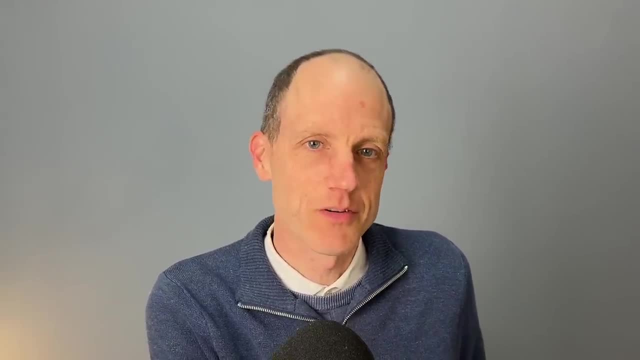 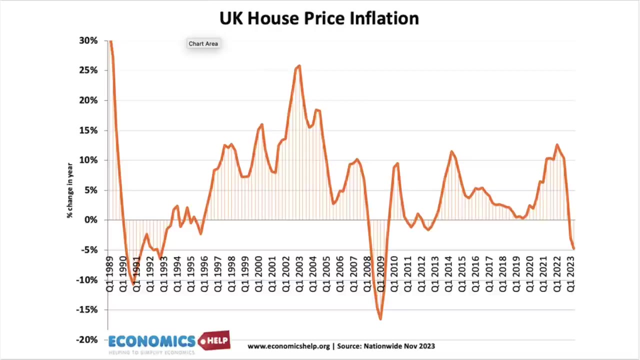 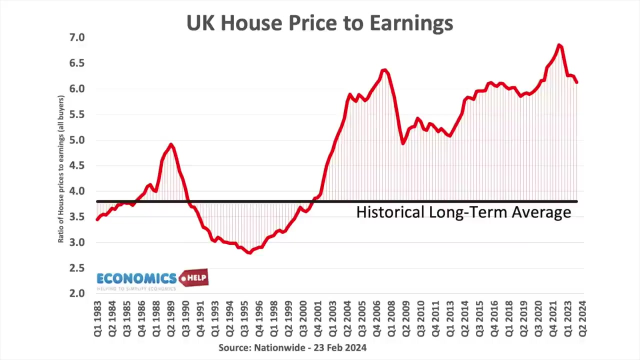 But it is immune from any kind of big house price falls. Well, house prices did fall in 2008 and the early 1990s, But I think that those hoping for a return to affordability levels last seen in the mid-90s were going to be disappointed, because only modest falls in house price to 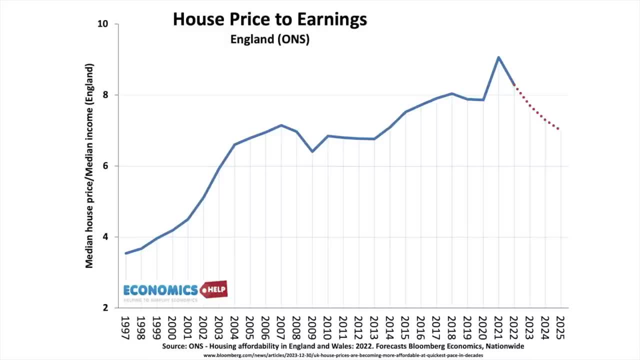 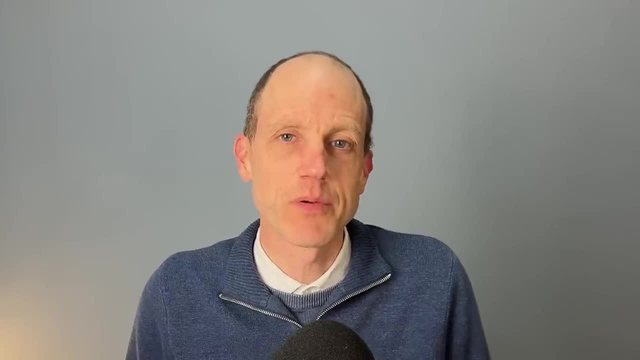 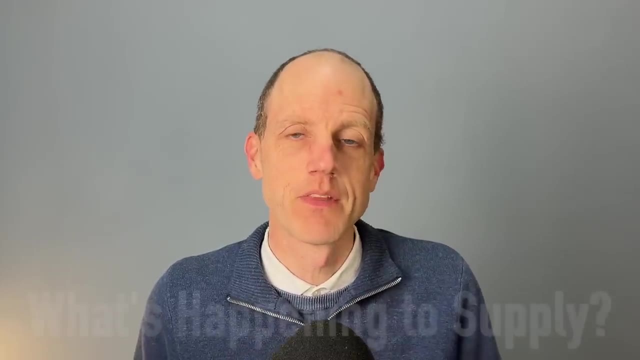 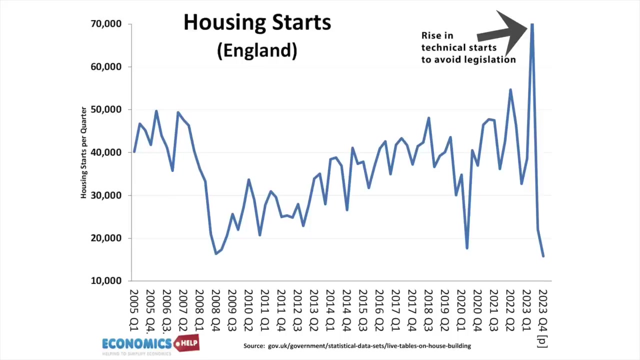 It's not just about income and interest rates, but the impact of wealth propping up house prices. So the result really is a two-speed housing market between those who can add wealth to buying a house and those who can't. Now, one damaging impact of the higher interest rates has been a cut to home building. The end. 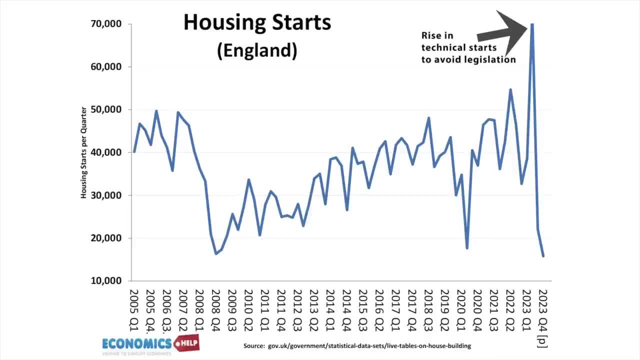 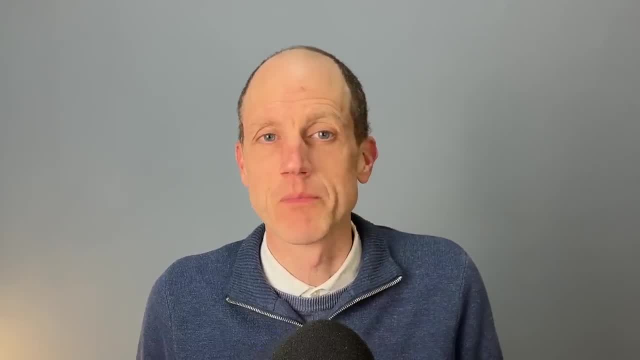 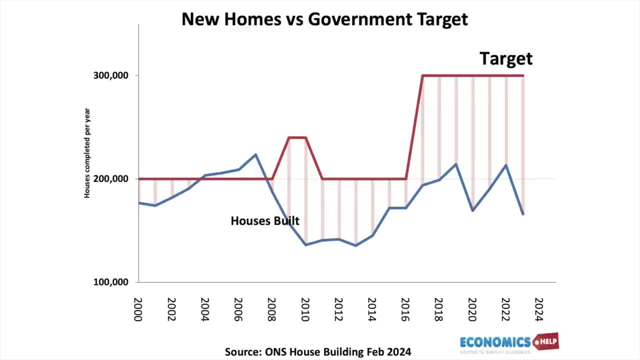 of last year saw many projects either cancelled or not finished. Combined with high inflation, higher wages, the higher interest rates have really made it difficult for home builders, who've pulled back from many projects. The result is that suppliers are expected to fall further away. 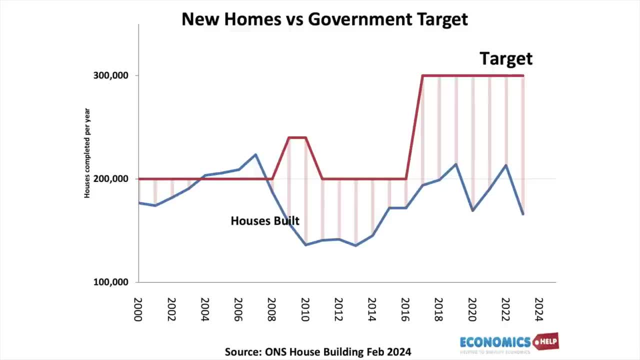 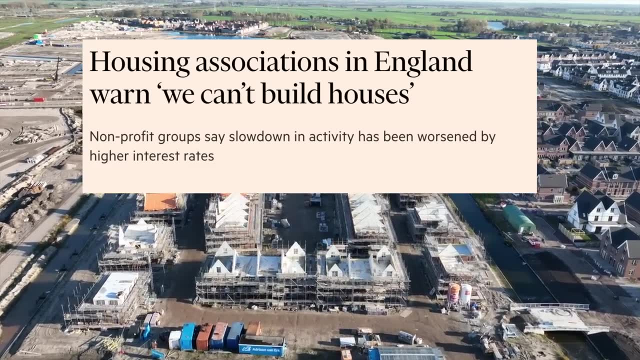 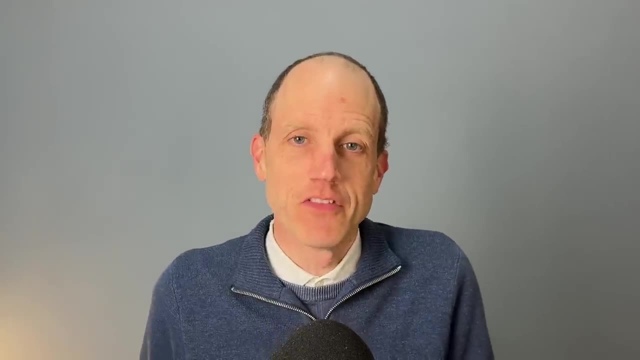 from government targets, and the impact is particularly acute in the affordable housing sector. Housing associations are warning that they can't manage to build projects and have left many projects half finished. The National Housing Federation warned that funding for affordable housing is now inextricably linked to interest rates because of a chain of economic changes. 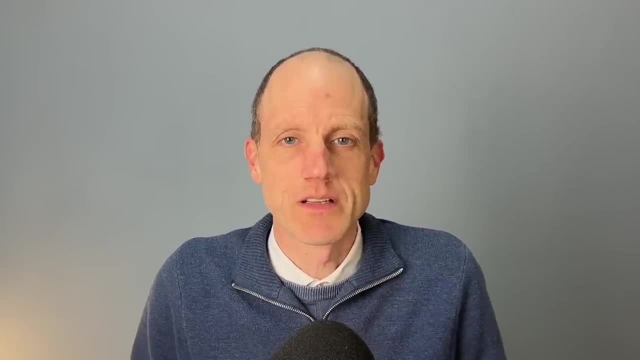 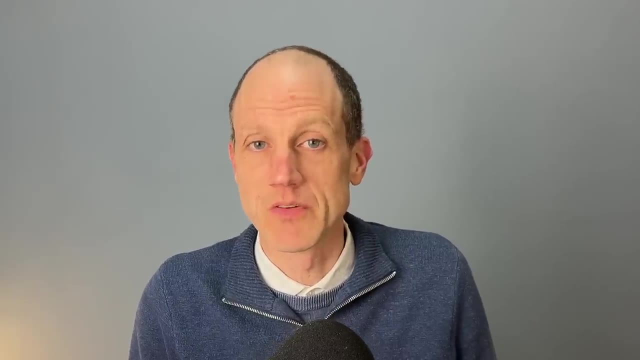 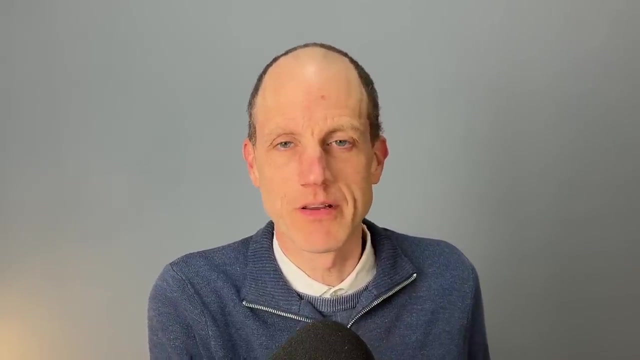 of a change in the funding model since the austerity of the 2010s, But this means with higher interest rates they can't build the 145,000 affordable homes that the UK really needs Now. Labour do have an ambitious plan to build many new homes if they're elected next year, but the past 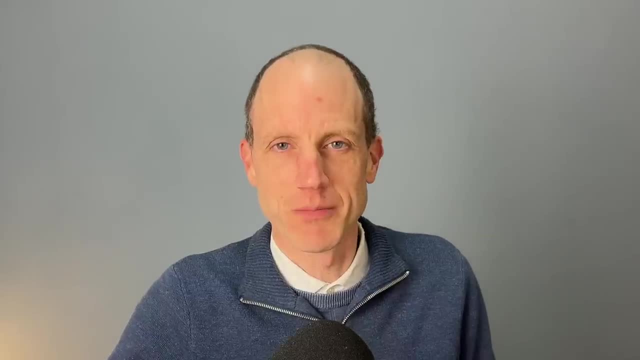 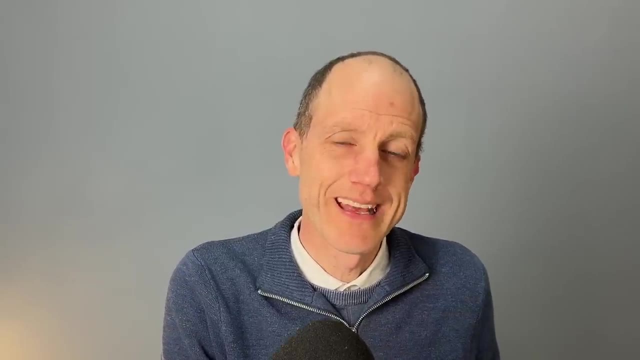 20 years do suggest that it's much easier to promise building housing than to actually deliver. And when the house building sector goes into recession and people stop working, it can be very difficult to get the building sector going again. It needs a degree of momentum. You can't just pick. 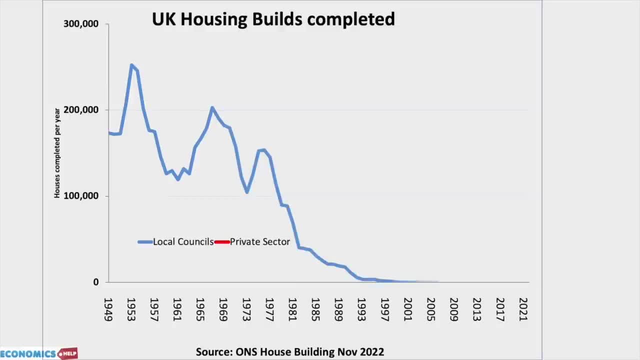 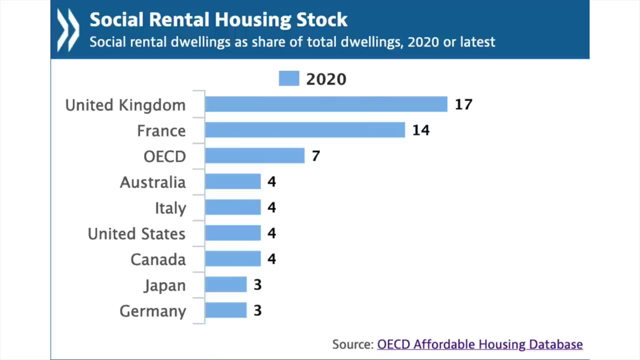 a number and say that's what we should build Now. in the post-war period, the UK was building much higher quantities of housing, in particular social housing. In fact, despite selling off one and a half million houses in the UK, the UK still has one of the highest rate of social housing in the OECD. 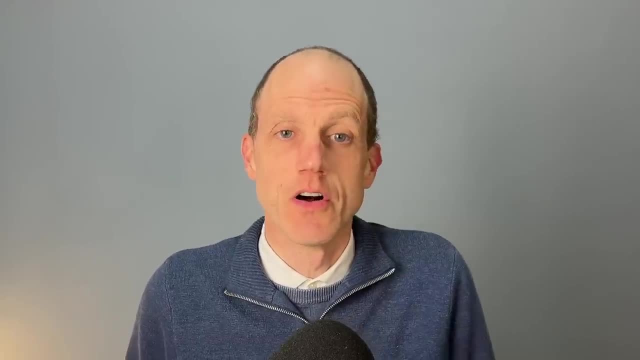 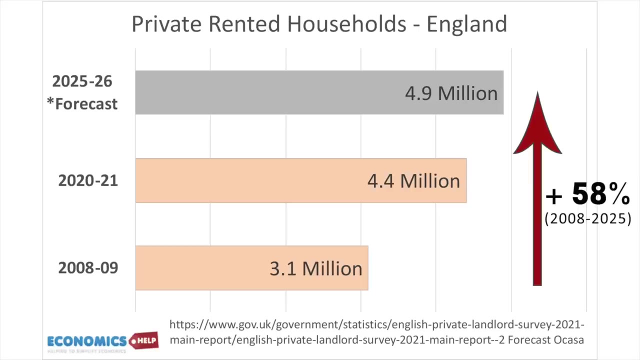 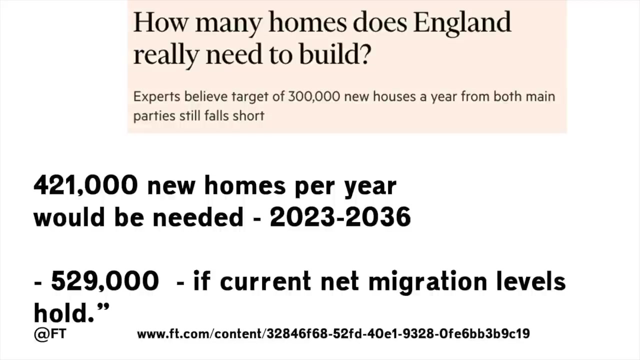 But the problem is that the UK is very much under development of the private rented sector. The loss of social housing and the rise in the population, partly due to high levels of immigration, have not been met. The FT report, according to some estimates, the UK actually needs 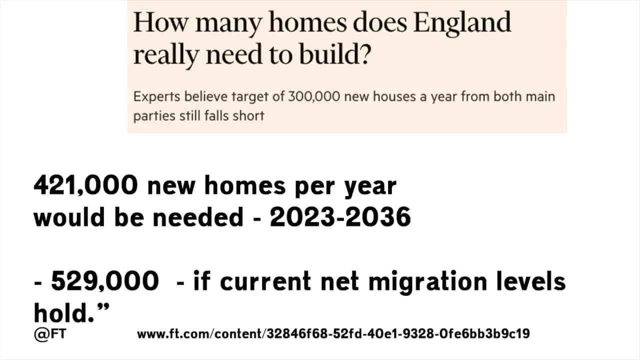 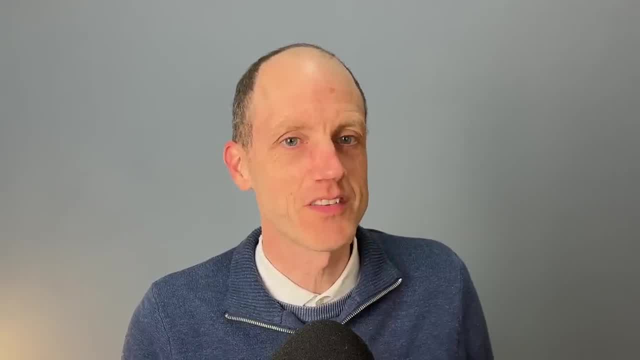 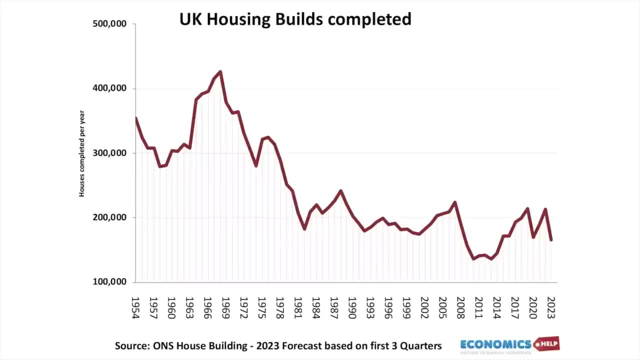 to build closer to 421,000 homes a year to catch up with the backlog, But currently the country is struggling to meet even much more modest needs. The UK is also struggling to meet the targets and it's really hard to see a return to 400,000 homes a year, which we only briefly saw in the late 1960s. 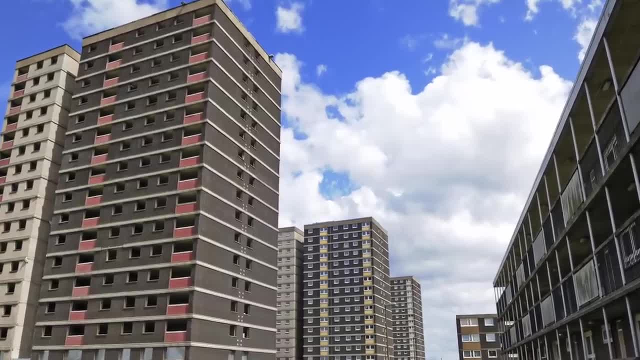 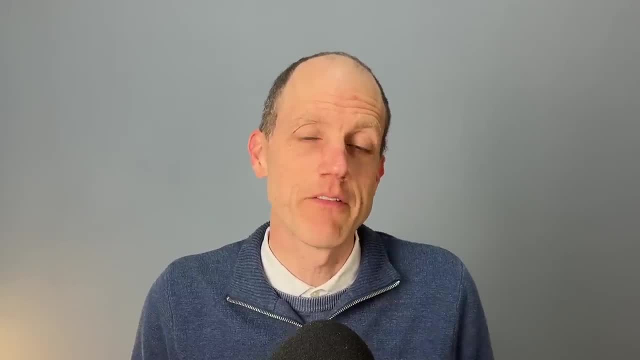 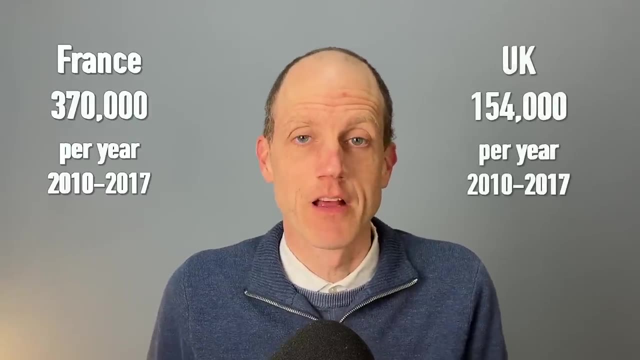 And that included many council tower blocks which later got demolished. Now again, in international comparison, France is a similar sized country and they have been building on average 370,000 homes between 2010-2017.. And in that period the UK built almost half that: 154,000. 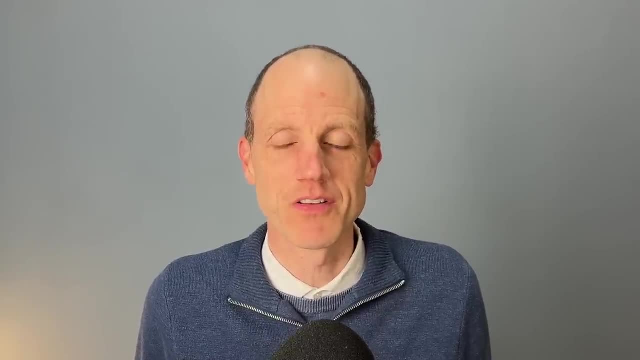 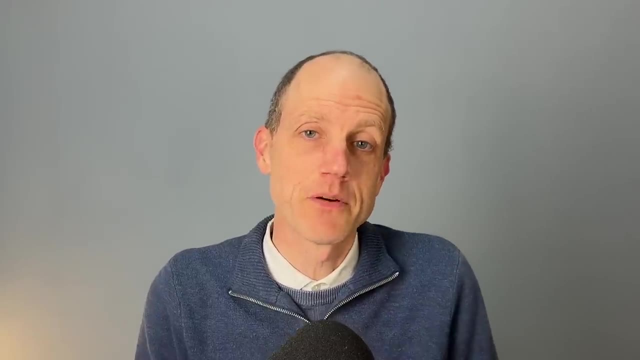 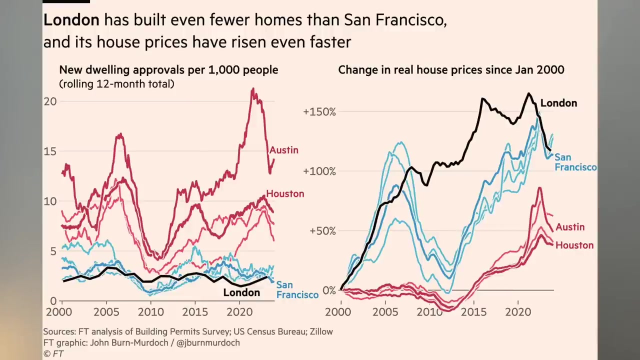 So you can see the difference in home building between two countries. Perhaps it's easier to build in France with more land, but whatever the case, France built a lot more And building does make a difference to house prices. London has seen relatively low rates of house building and the highest rise in prices. Texas, which admittedly 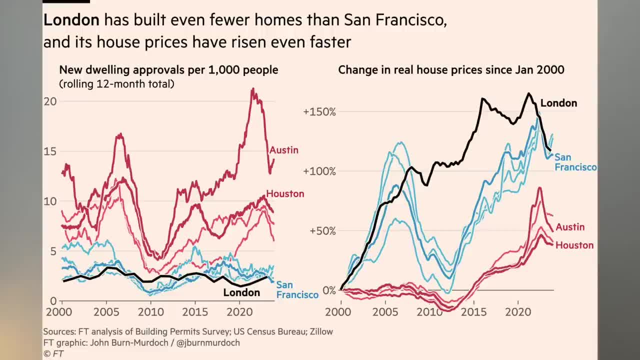 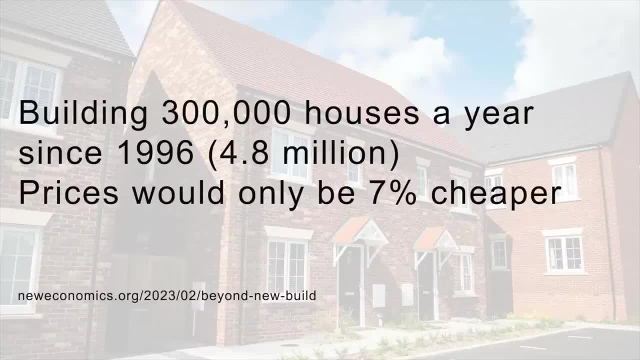 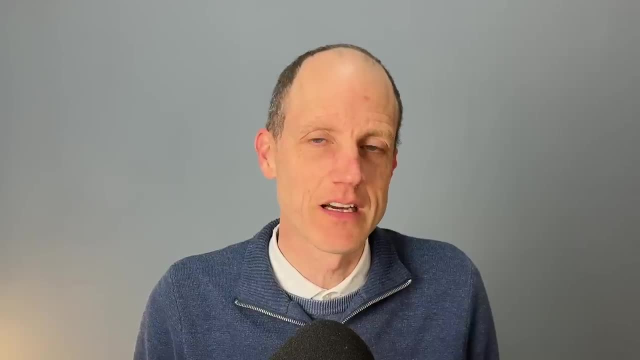 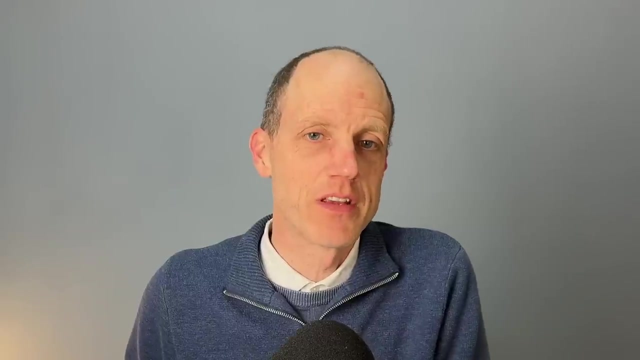 has much more space, has avoided excess price rises by being able to build more. Now it is a fair point to say that sometimes supply is blamed too much for high prices. Certainly, the boom in house prices since 2009 was to a large extent due to the ultra low interest rates, And some claim that the UK is